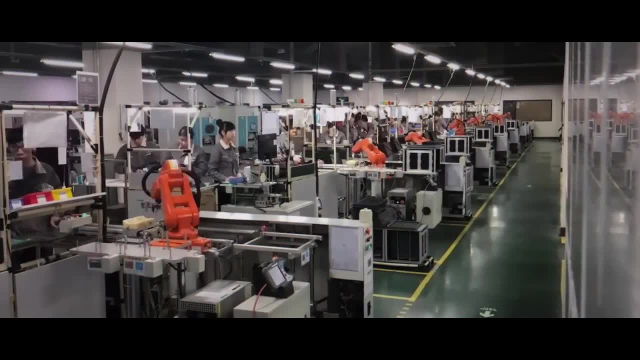 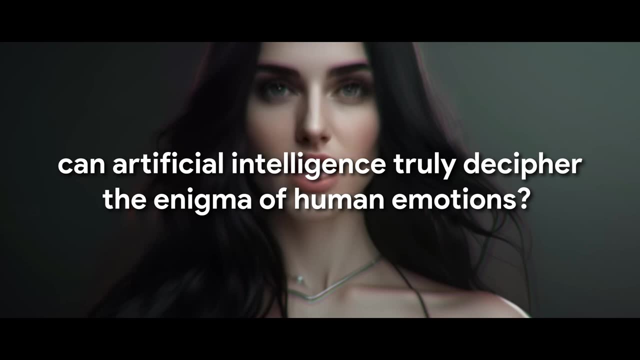 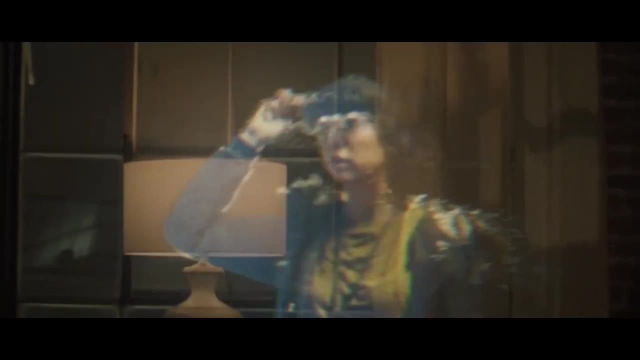 Picture this: a world where machines don't just compute but also sense and feel. The question is: can artificial intelligence truly decipher the enigma of human emotions And, if so, how will it redefine our connection with technology In today's captivating exploration? 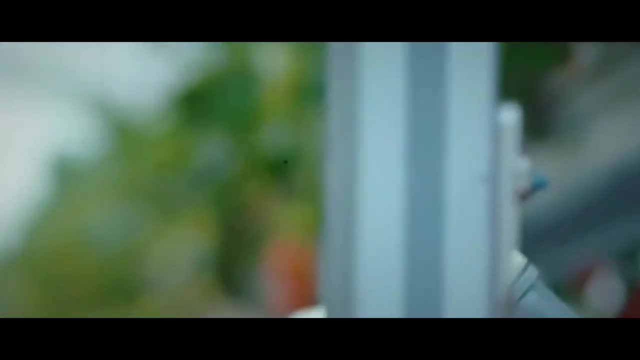 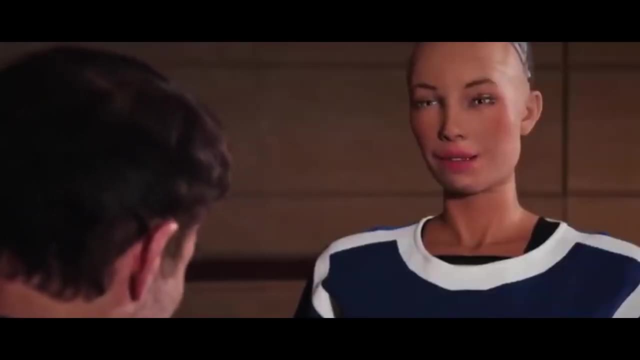 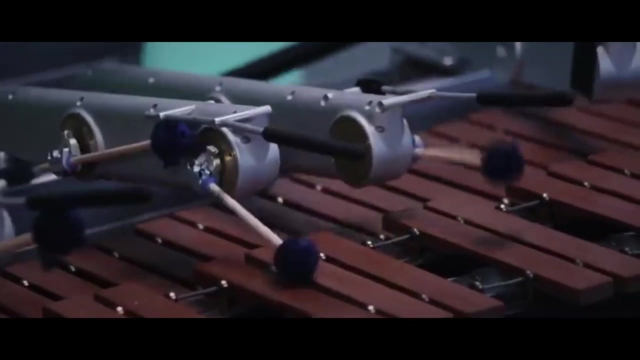 we'll navigate the emotional labyrinth that separates human minds from the ever-advancing realm of AI. Prepare to challenge your understanding of emotional intelligence as we unravel groundbreaking insights from neuroscience, leaving you to ponder the true potential of AI in grasping human emotions. 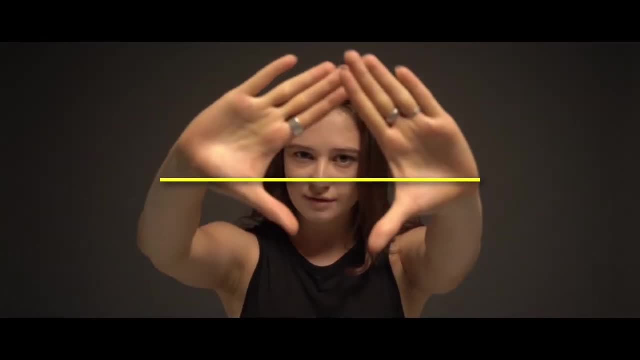 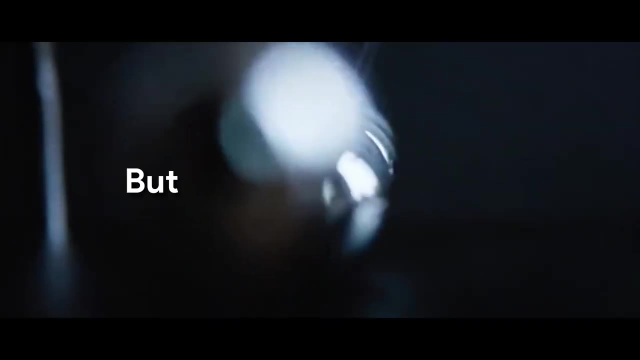 Number 1 – The Definition of Human Emotion. Human emotions, those intricate and powerful feelings, have captivated and puzzled us for centuries. But what are they really At their core? emotions are complex psychological emotions. But what are they really At their core? emotions are complex, psychological and. 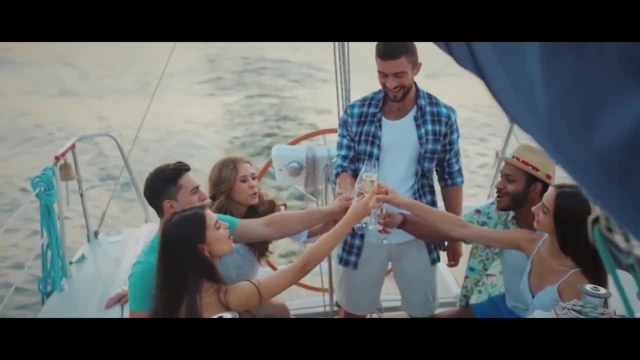 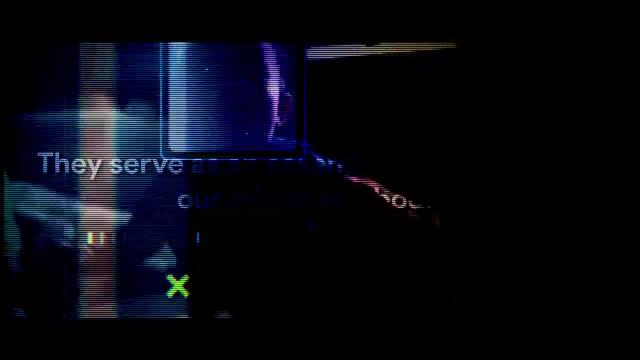 emotional emotions. But what are they really? At their core, emotions are complex psychological and physiological responses to specific situations, experiences or even thoughts. They serve as an essential bridge between our minds and bodies, helping us navigate through life's challenges and triumphs. 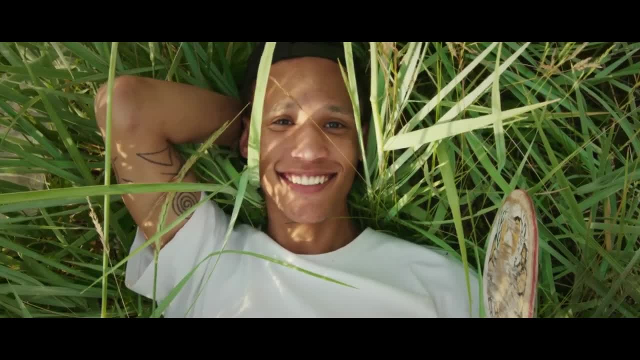 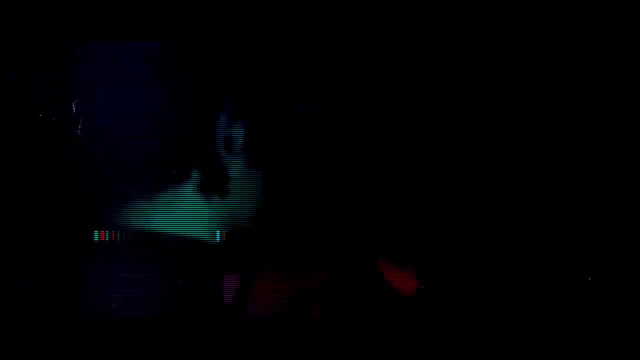 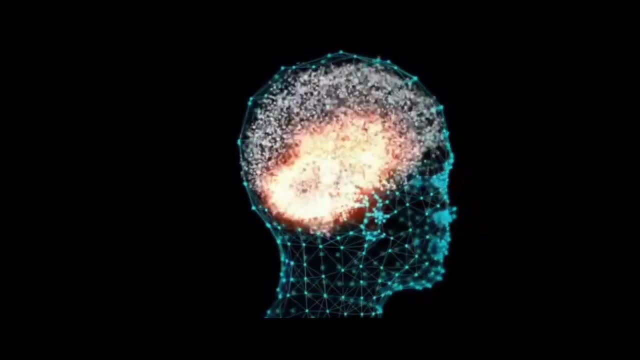 Think about the last time you felt a surge of happiness after receiving an unexpected compliment, or the all-consuming anger bubbling inside you during a heated argument. These emotional responses are guided by a fine-tuned interplay between our brain, nervous system and hormones working together in a delicate dance. 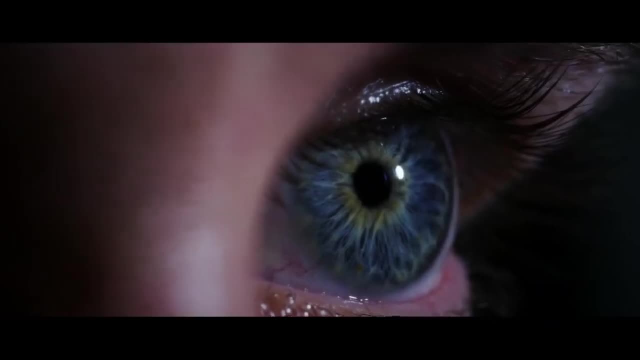 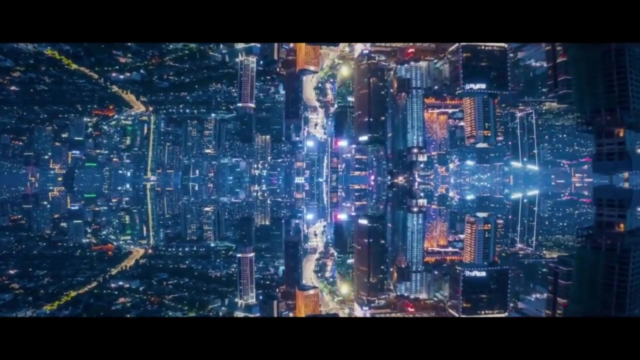 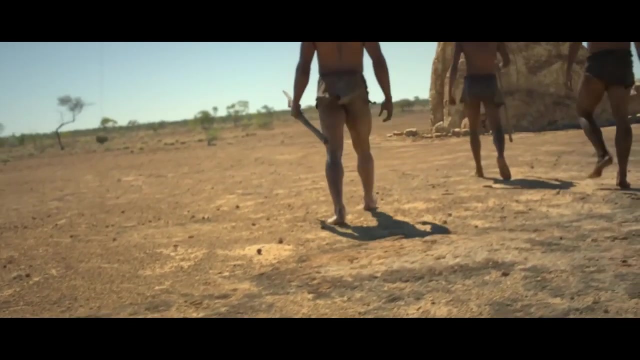 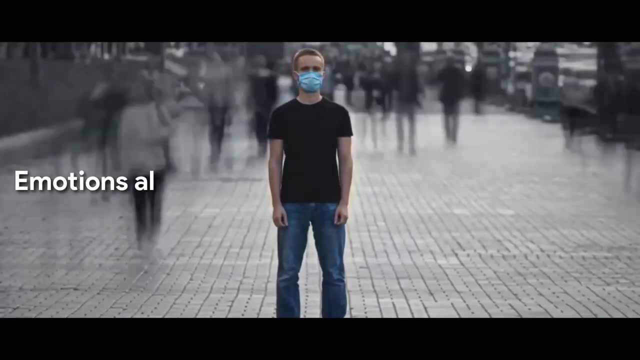 Scientists have identified a range of basic emotions, such as joy, sadness, anger, fear and surprise, that are universally experienced across cultures. These emotions, deeply rooted in our evolutionary history, have helped our ancestors survive by preparing their bodies for action, like running away from a predator or protecting their offspring. Emotions also play a. 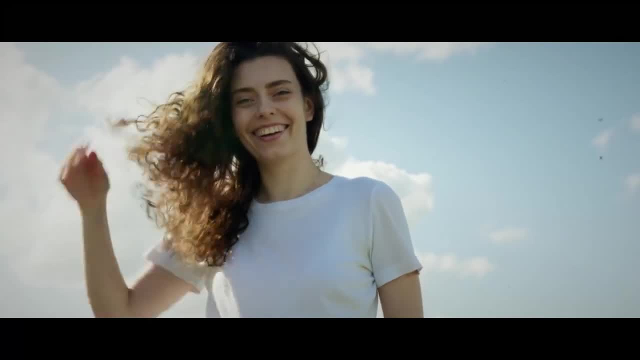 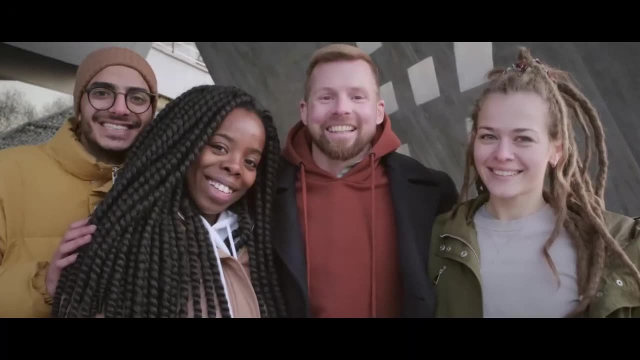 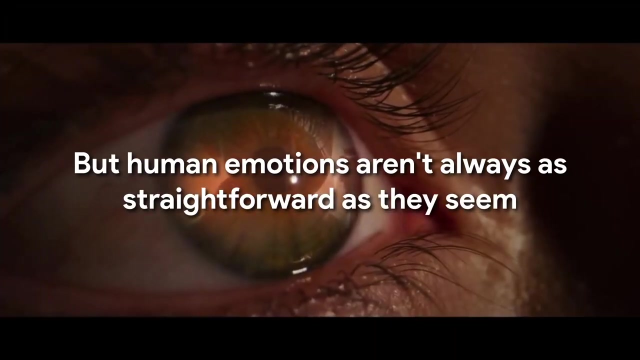 crucial role in communication. A warm smile, a furrowed brow or a quivering voice can convey our inner feelings without the need for words, strengthening our social bonds and enabling us to empathize with one another. But human emotions aren't always as straightforward as they seem. 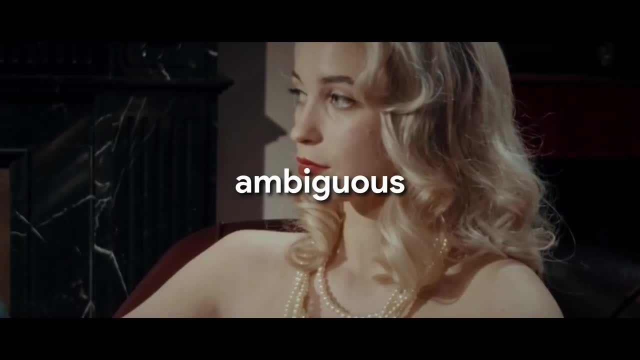 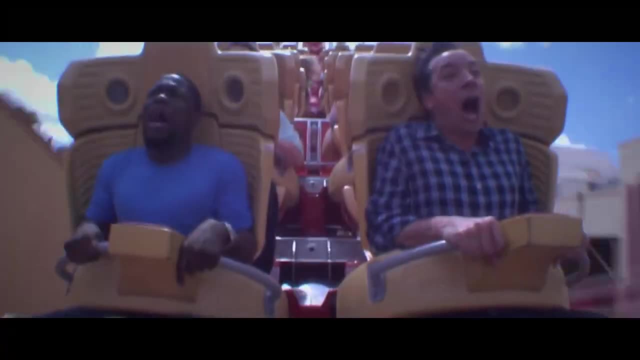 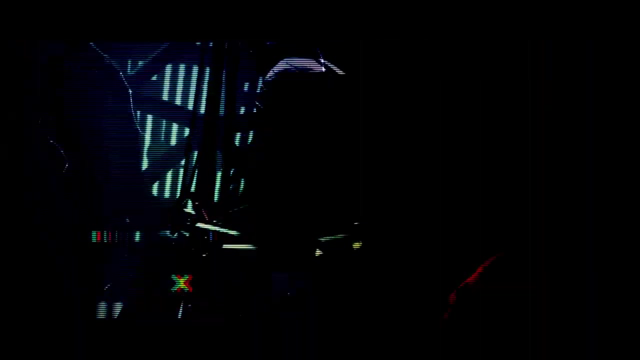 They can be fleeting or enduring, clear or ambiguous, and can even blend together to create complex feelings like bittersweet nostalgia or the thrill of anticipation. This rich emotional tapestry is what makes us uniquely human, And yet it's also what leaves us wondering if artificial intelligence could ever truly grasp its intricacies. 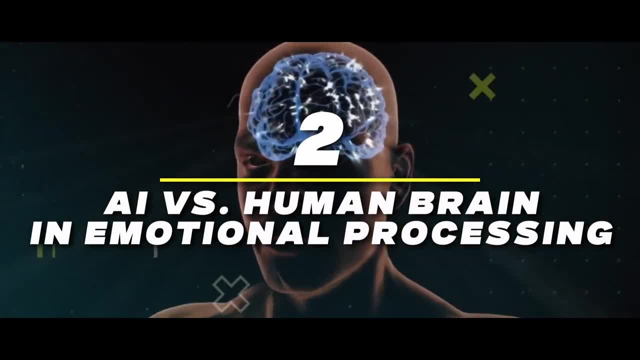 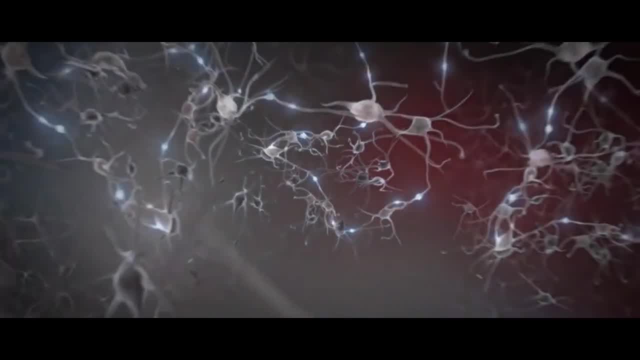 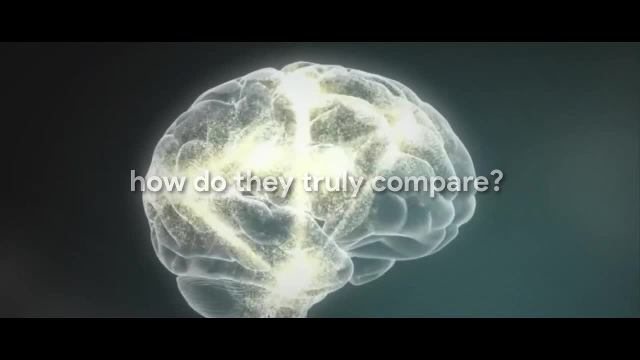 Number 2. AI vs Human Brain in Emotional Processing. AI and the human brain: two vastly different worlds, yet both capable of incredible feats. But when it comes to emotional processing, how do they truly compare? Are we witnessing an epic clash of intelligences or is this simply an apples-to-oranges? 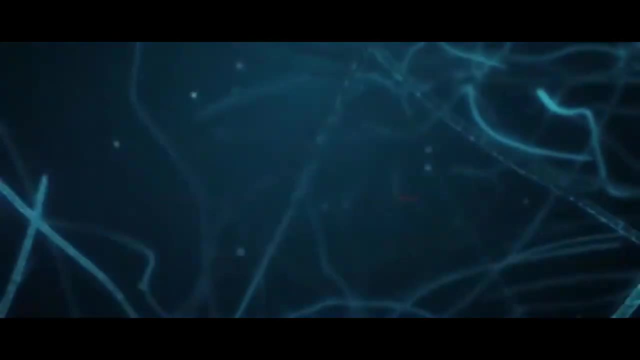 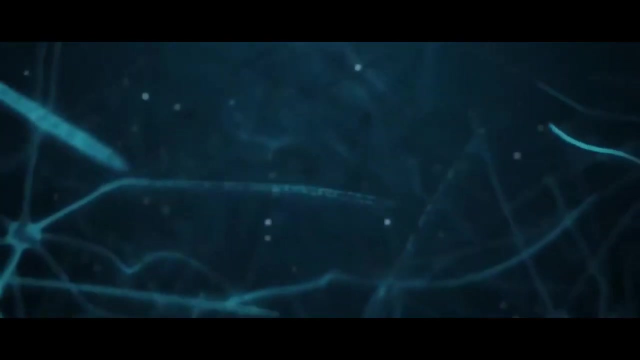 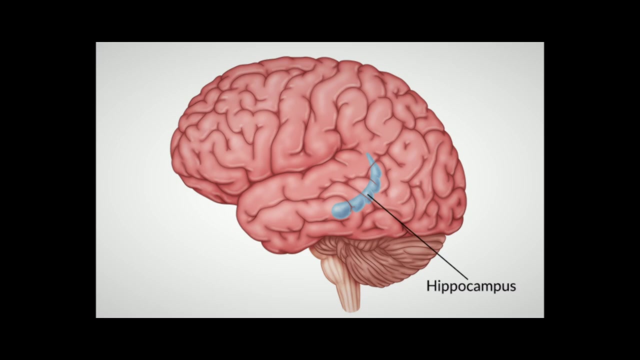 comparison. The human brain is a remarkable organ with over 100 billion neurons firing away, shaping our thoughts, actions and emotions. Emotional processing is nestled within its intricate networks governed by regions like the amygdala, hippocampus and prefrontal cortex. 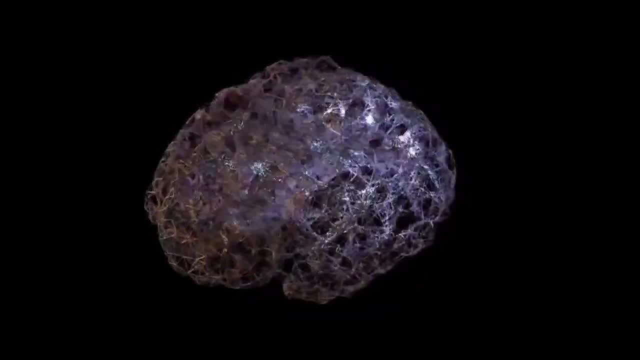 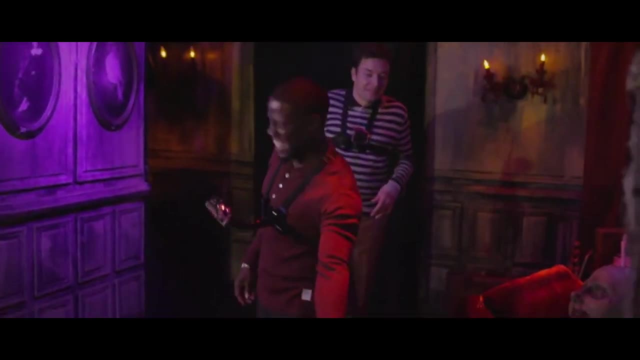 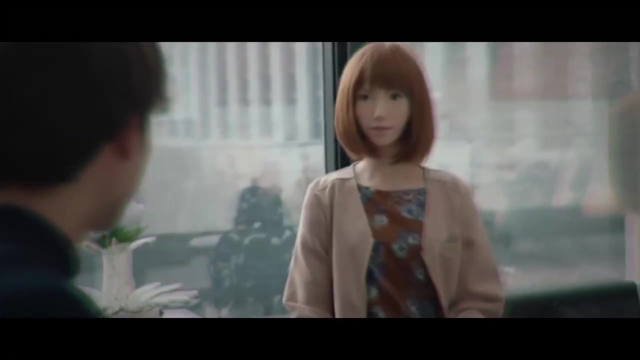 These areas collaborate to evaluate situations, generate feelings and guide our reactions: From the heartwarming embrace of a loved one to the spine-chilling suspense of a thriller, our brains decode these scenarios and conjure up the emotions we experience. AI, on the other hand, is a product of human ingenuity, designed to mimic aspects of human. 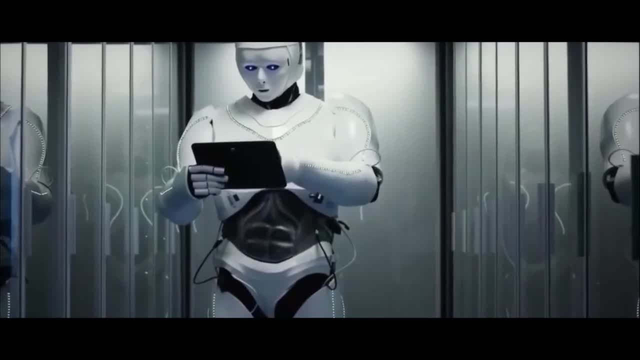 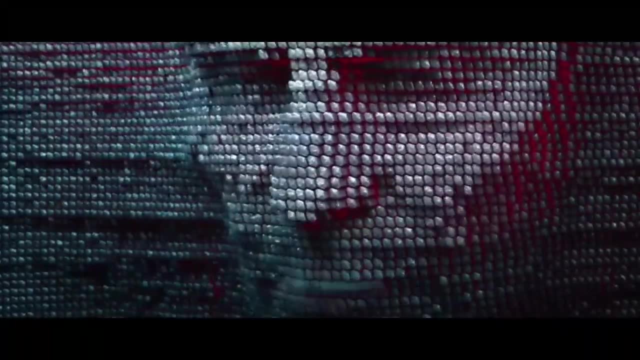 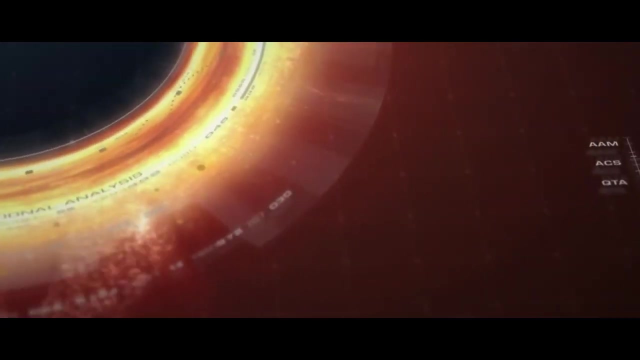 cognition. While it lacks the organic architecture of the brain, AI compensates with powerful algorithms and vast data sets. In the realm of emotional processing, AI leverages techniques like facial recognition, sentiment analysis and natural language processing to identify and interpret emotions. 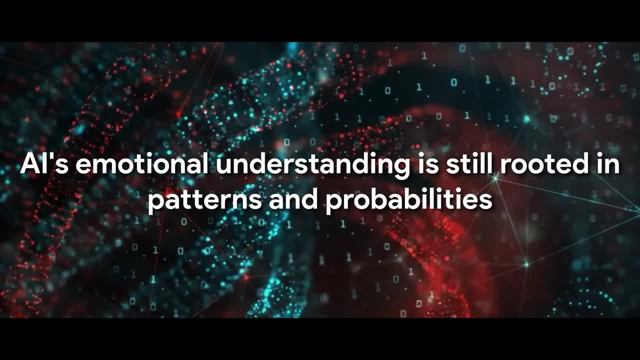 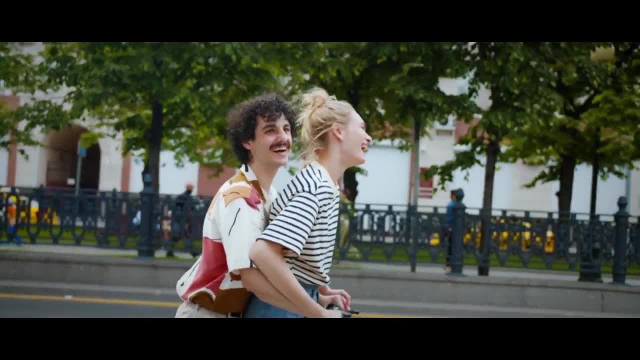 However, AI's emotional understanding is still rooted in patterns and probabilities, rather than the experiential and instinctive nature of human emotional processing. So are we witnessing a true rivalry between AI and the human brain, or is it more of a conflict? 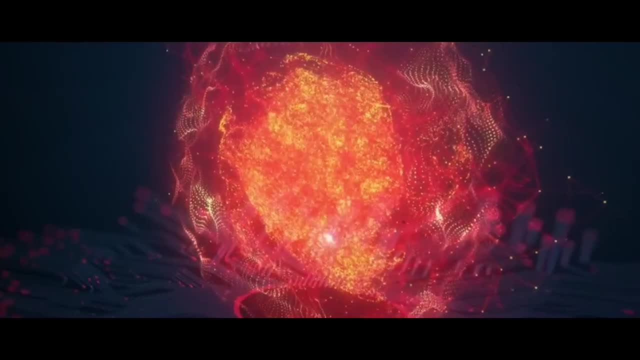 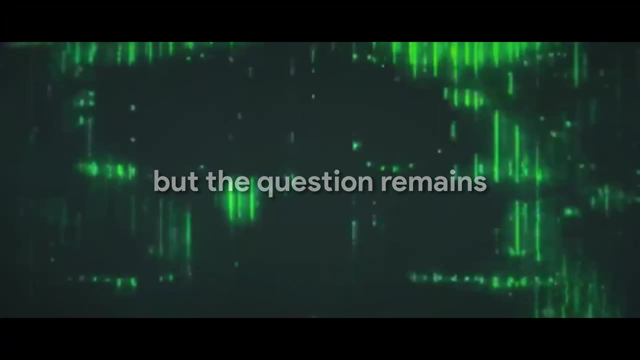 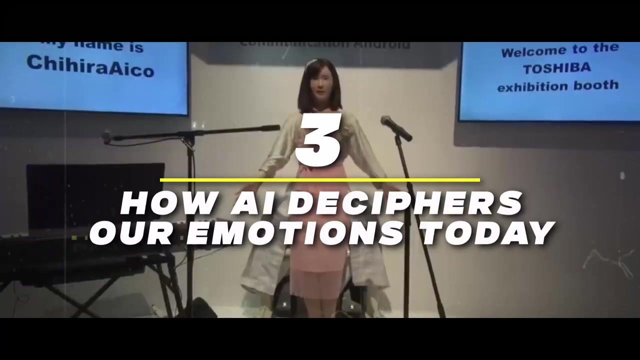 This is a fascinating collaboration. As AI continues to advance, it may learn to decipher the nuances of human emotions more effectively, but the question remains: can it ever truly replicate the authentic, deeply personal experience of human emotional processing? Number 3 – How AI Deceptifers Our Emotions Today. 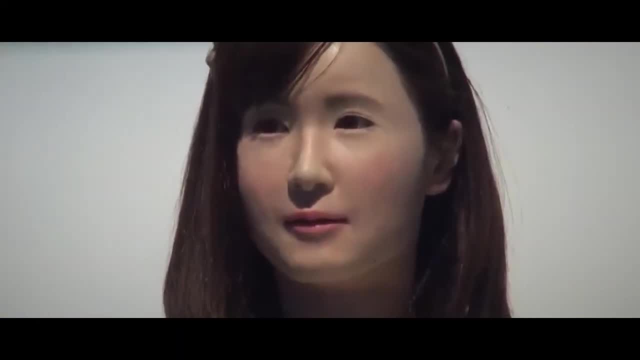 With their digital prowess, artificial intelligence ventures into the world of emotions, decoding them with remarkable, albeit impossible because of new technology. AI is going to test the emotions and it will decide if they will ever go backward and, if they will go forward, whether it will be to 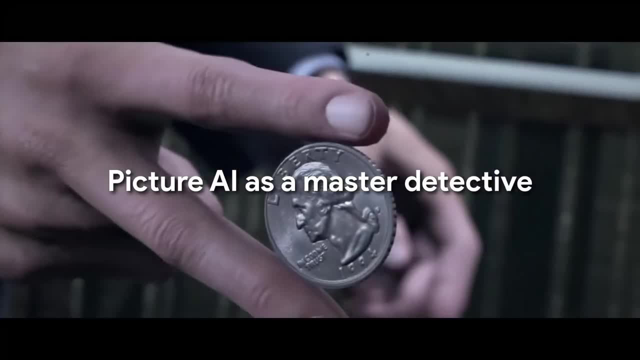 go forward or not. AI is looking for a new way to move the emotions and understanding them If they are to be forged. we need more time to think about how to overcome the challenges that we face with AI. perfect precision Picture AI as a master detective armed with an array of tools to 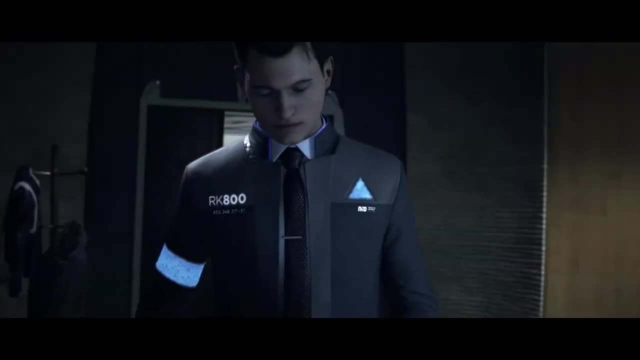 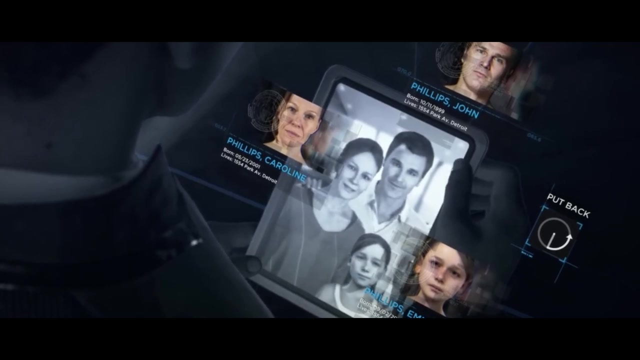 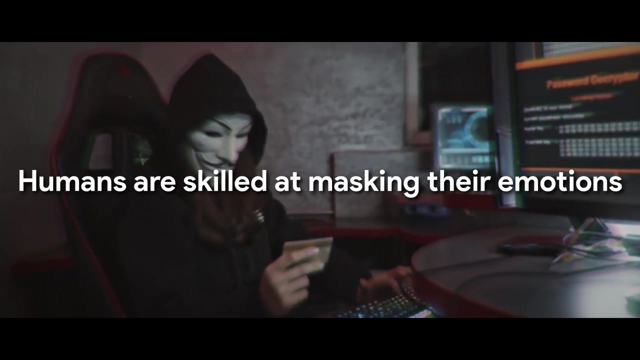 deduce our emotional states. One such tool is facial recognition, analyzing the subtle contours of our expressions to identify emotions like joy, sadness or surprise. But beware, for appearances can be deceiving. Humans are skilled at masking their emotions and the context of the situation. 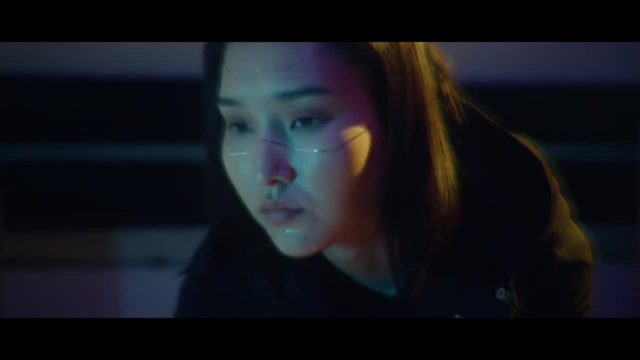 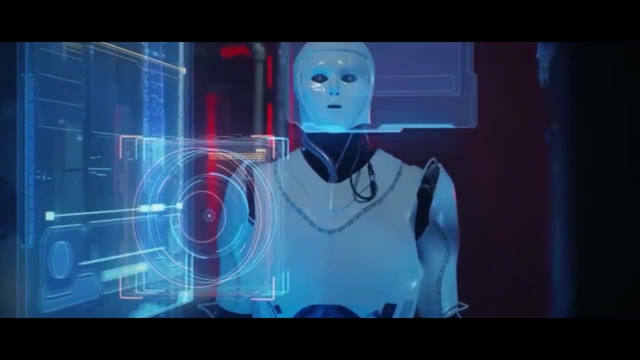 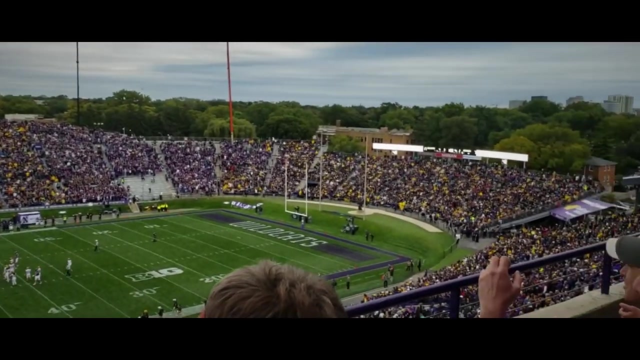 may sometimes elude even the sharpest AI. Another instrument in AI's emotional toolbox is sentiment analysis. By scrutinizing the words we use and the tone of our voice, AI can gauge our feelings with surprising accuracy From the cheerful tweets of a sports fan. 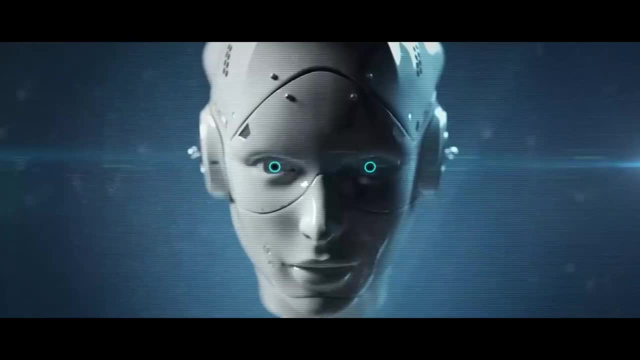 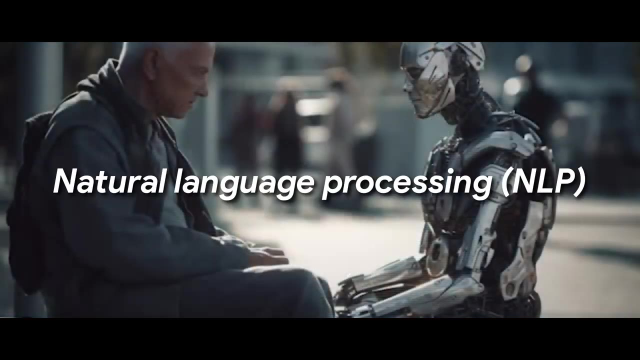 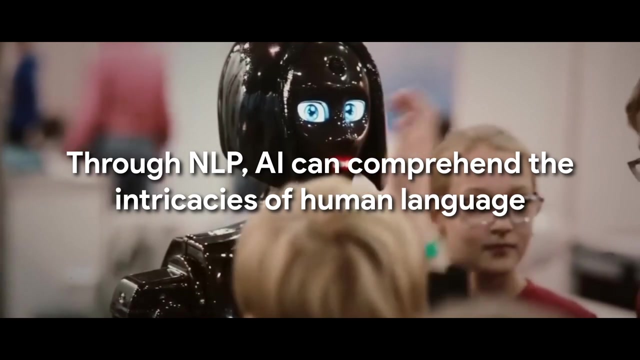 to the melancholic lyrics of a heartbroken poet. AI dissects these verbal cues, searching for emotional fingerprints. Natural language processing- NLP- also plays a crucial role in AI's emotional understanding. Through NLP, AI can comprehend the intricacies of human. 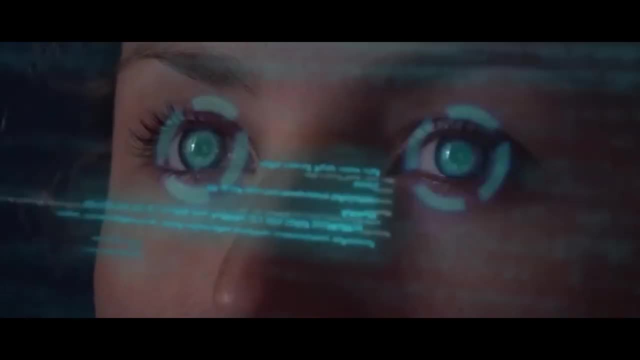 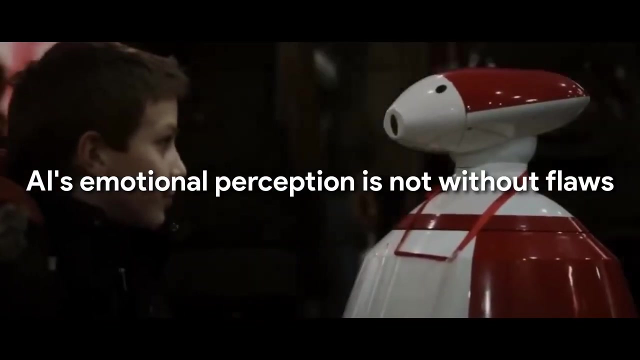 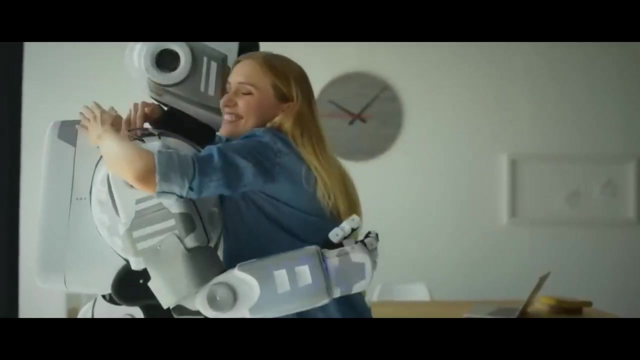 language, identifying emotional cues hidden within our phrases, slang and metaphors. Despite these impressive skills, AI's emotional perception is not without flaws. Machines still struggle with context and the ever-changing nature of human emotions, while AI's progress in deciphering our feelings is undoubtedly extraordinary. 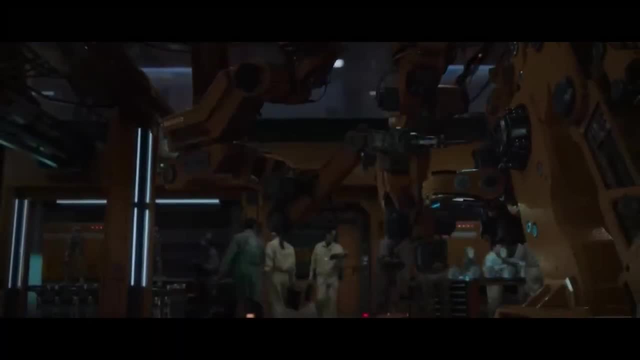 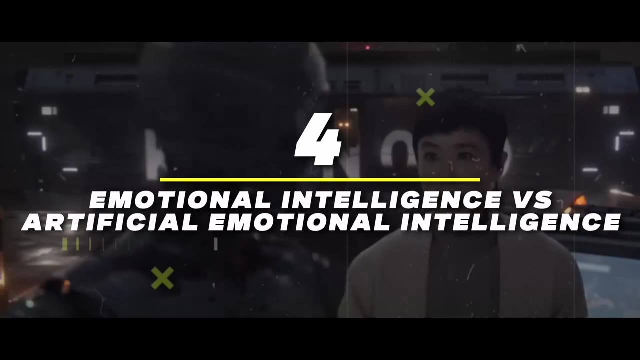 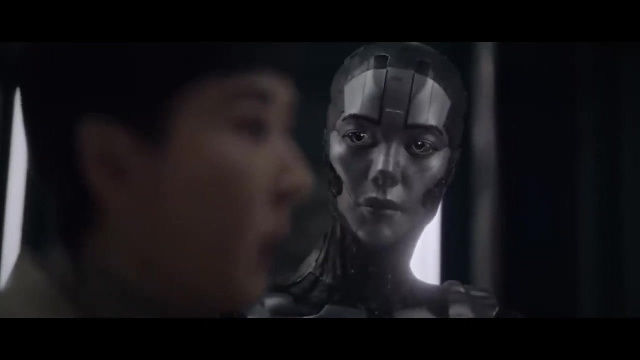 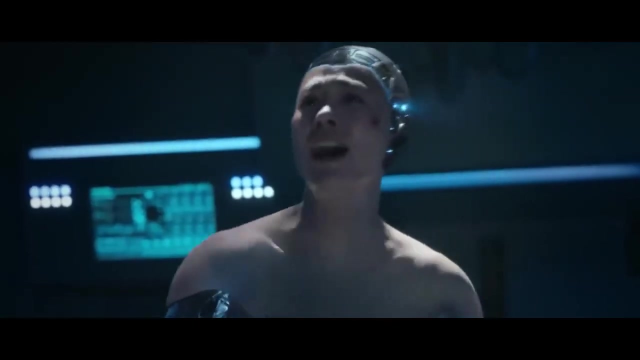 We must ask ourselves: can it ever truly grasp the elusive essence of human emotions? The answer may surprise you. Number 4. Emotional Intelligence vs Artificial Emotional Intelligence. As we venture deeper into the world of emotions, a fascinating face-off emerges: Emotional Intelligence EI vs Artificial Emotional Intelligence- AEI. But are they true? 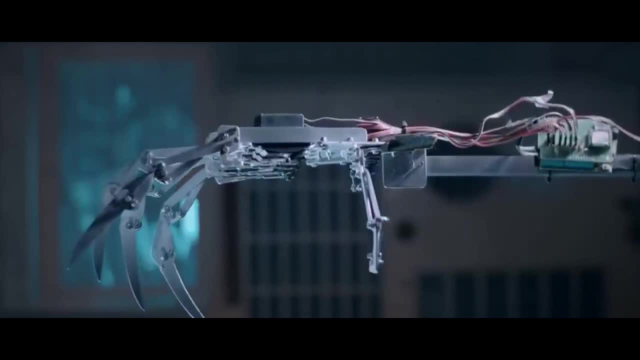 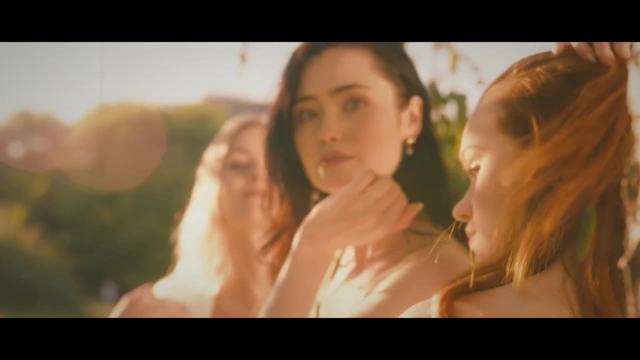 adversaries or are they just a part of the game? We must ask ourselves. can it ever truly grasp the depth of our emotions? No, For the most part, there's no doubt that we are living in the world of emotions. Emotional intelligence, an innate human trait, encompasses our ability to recognize, understand. 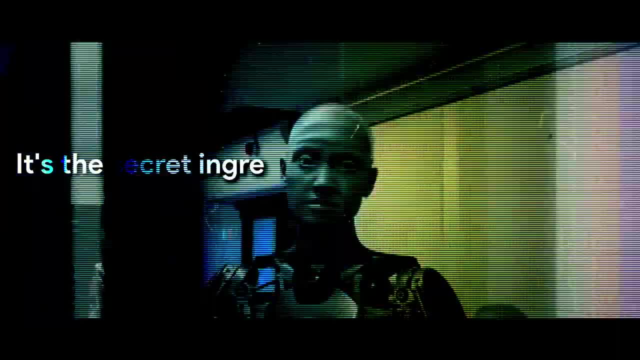 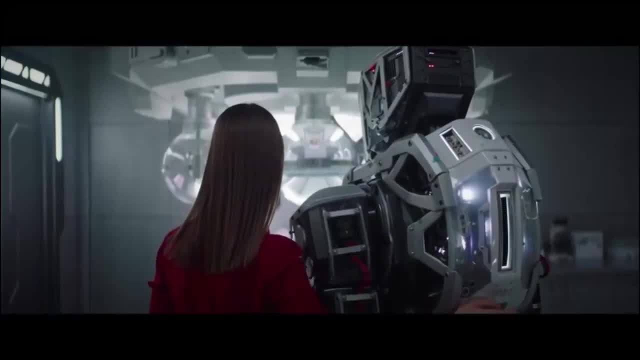 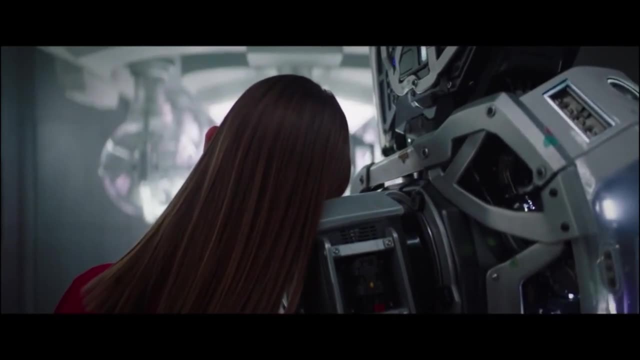 and manage our own emotions and those of others. It's the secret ingredient that enables empathy, compassion and effective communication. Imagine an empathetic friend who knows when to offer a shoulder to cry on, or the charismatic leader who inspires and motivates their team. 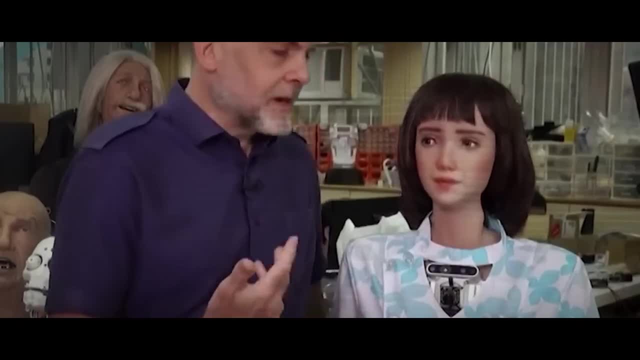 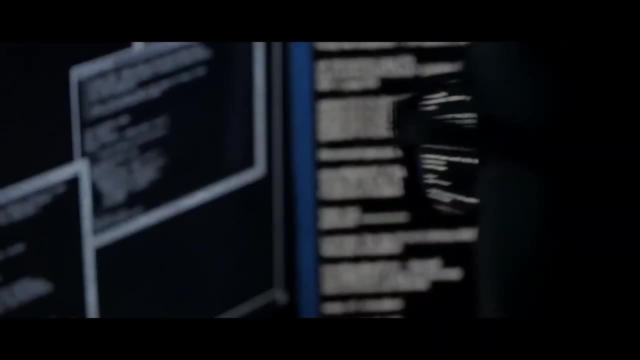 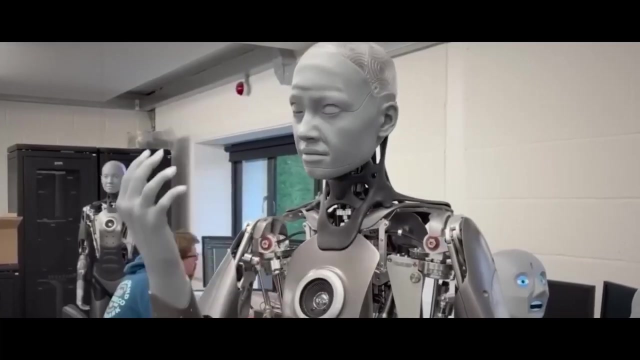 That's EI in Act Edition. Artificial emotional intelligence, on the other hand, represents AI's attempt to emulate this unique human ability. AEI, equipped with advanced algorithms and vast datasets, strives to interpret and respond to our emotions appropriately. Think of a customer service chatbot. 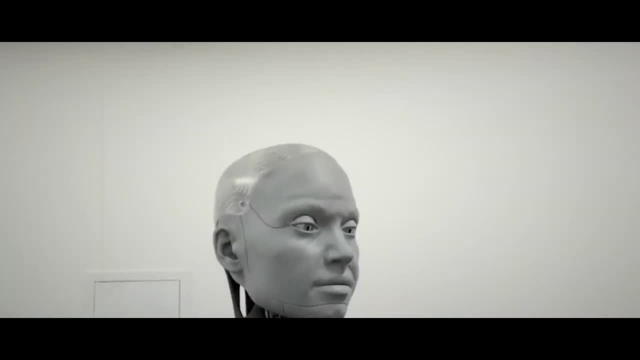 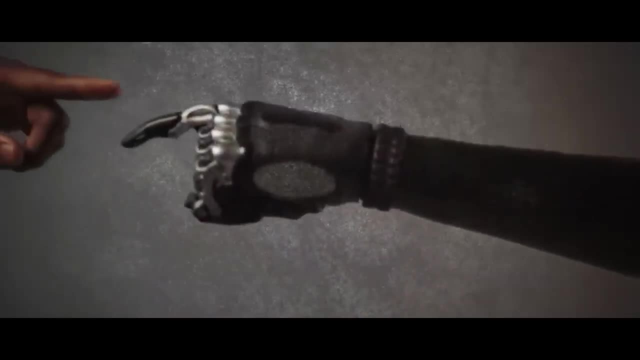 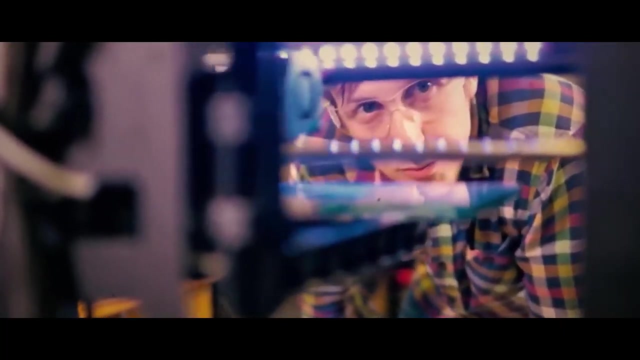 that detects your frustration and tries to soothe your concerns, or an AI therapist that identifies the subtle signs of depression. That's AEI making strides. Despite their differences, EI and AEI are not true rivals, but rather complementary forces in the pursuit of understanding emotions, While human EI boasts intuition experience. 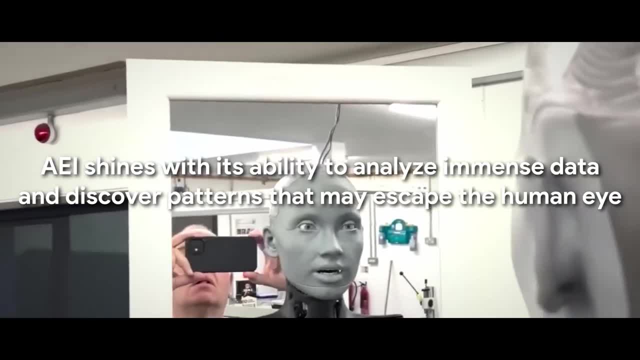 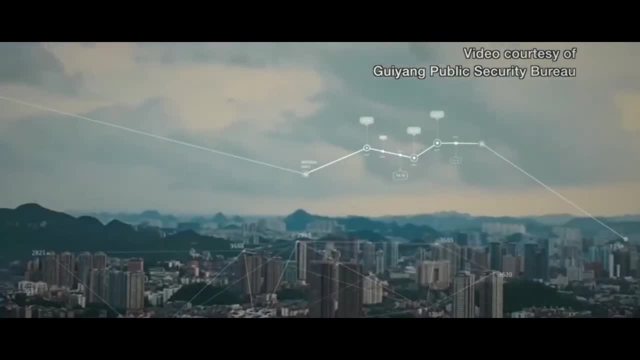 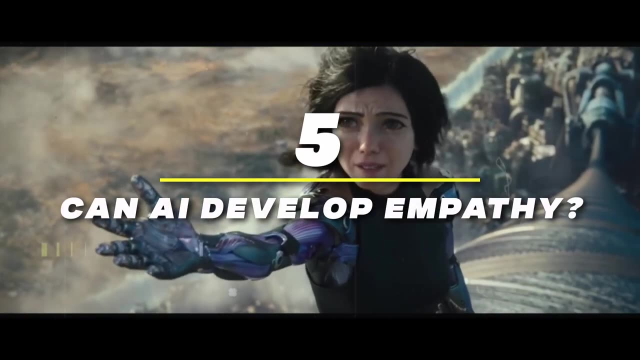 and the power of empathy. AEI shines with its ability to analyze immense data and discover patterns that may escape the human eye. Together, they can forge a powerful alliance that will enable them to achieve their goals, and achieve their goals. 5. Can AI Develop Empathy? Can AI develop empathy? 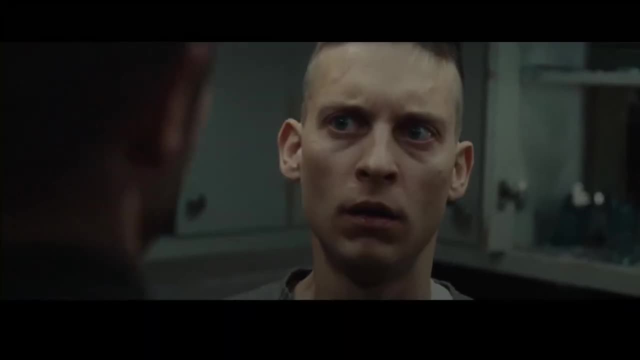 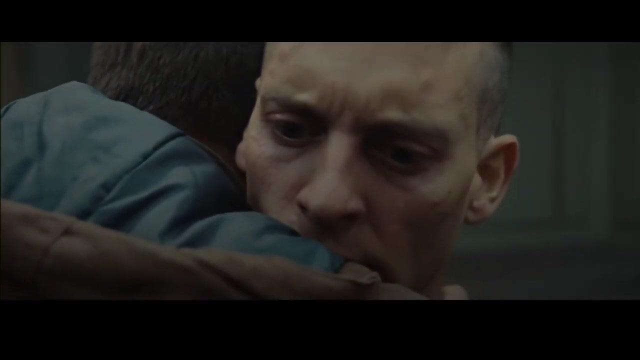 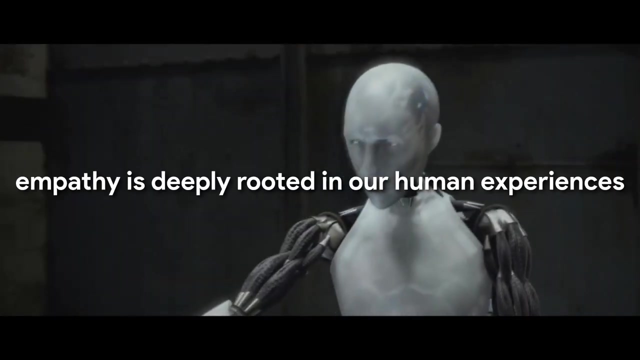 that quintessential human quality that enables us to share and understand the feelings of others. At first glance, the idea of empathetic AI may seem far-fetched, like something straight out of a science fiction novel. After all, empathy is deeply rooted in our human experiences. 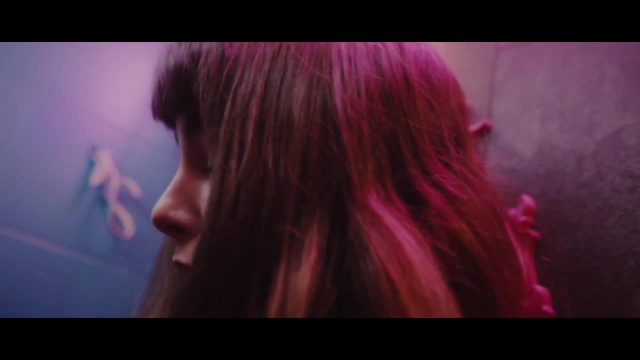 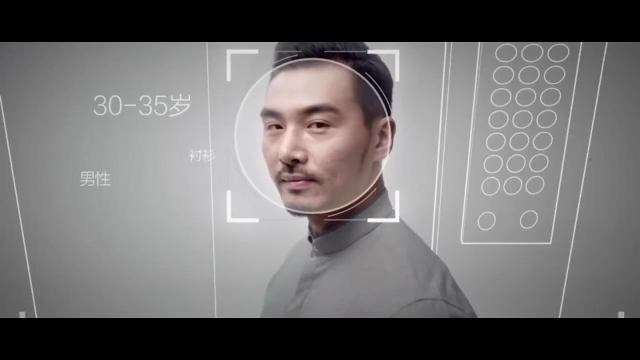 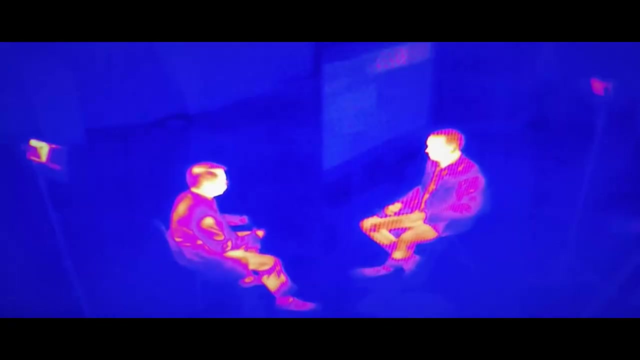 emotions and relationships, Aspects that machines lack by nature. However, AI has been making strides in mimicking empathy, thanks to advanced algorithms and an ever-growing understanding of human emotions. Consider AI-powered chatbots that can detect and respond to our emotional cues. 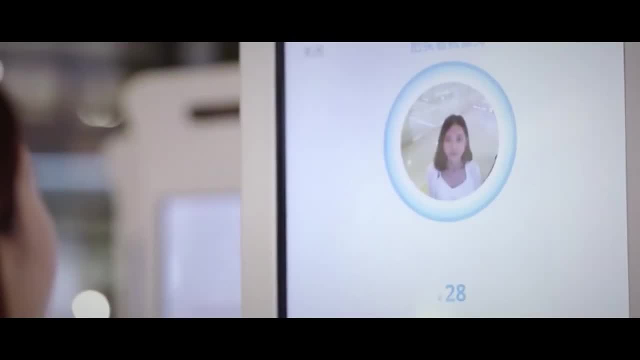 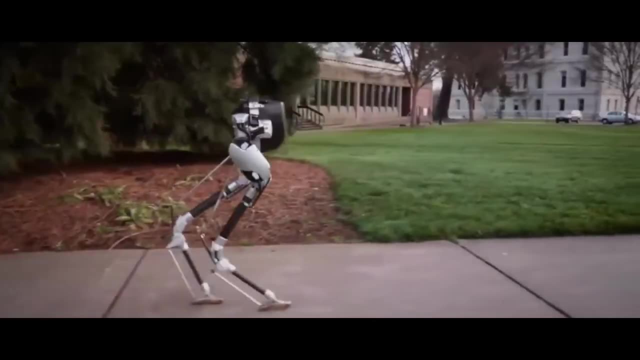 offering comforting words or helpful suggestions based on our feelings. These digital companions can create the illusion of empathy, but is it genuine? 6. The Crux of the Matter: The crux of the matter lies in the difference between simulating empathy and truly experiencing it. 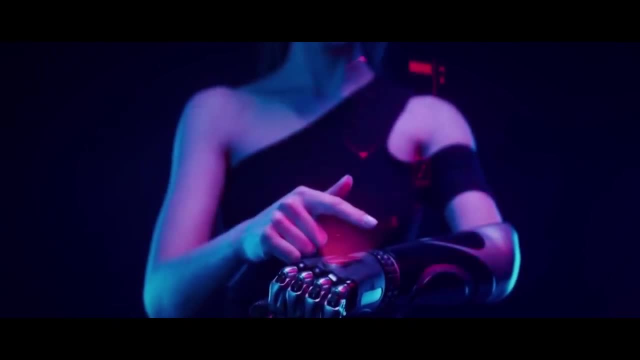 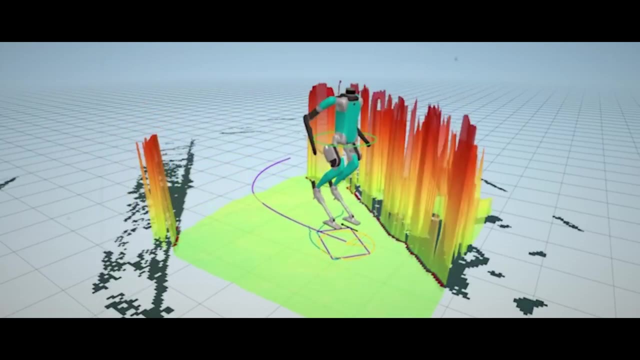 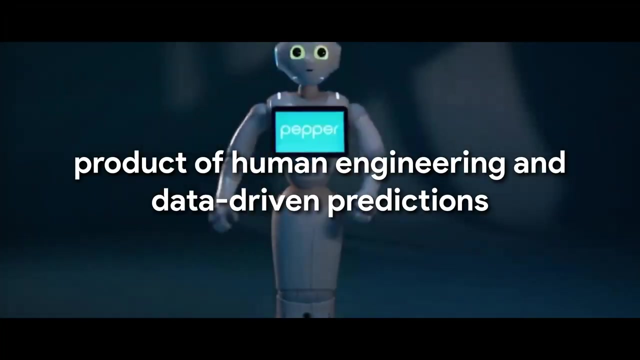 While AI can be programmed to recognize emotions and respond accordingly, it does so based on patterns and probabilities rather than genuine emotional understanding. The AI's empathy is, in essence, a carefully crafted illusion, a product of human engineering and data-driven predictions. So can AI truly develop empathy? 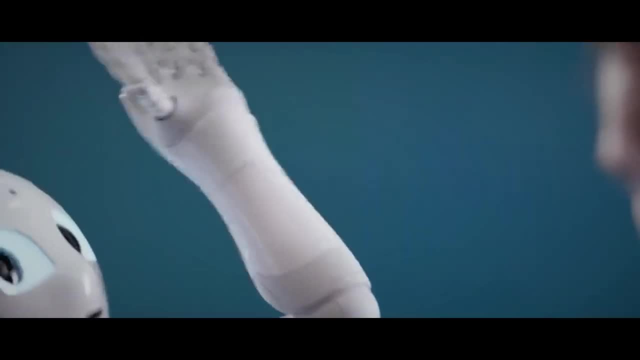 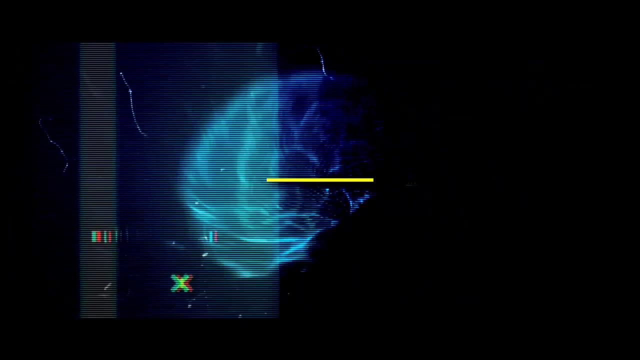 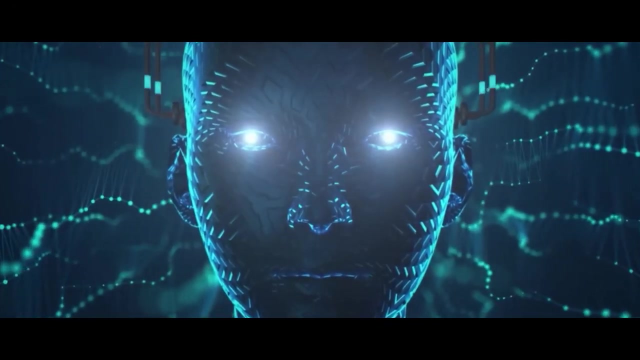 7. Can AI Develop Empathy? For now, it seems that true empathy remains a uniquely human trait, one that arises from our lived experiences and emotional connections. 6. Neuroscience: The Secret Weapon for AI's Emotional Leap. In the quest for AI's emotional leap, an unexpected ally emerges: Neuroscience. 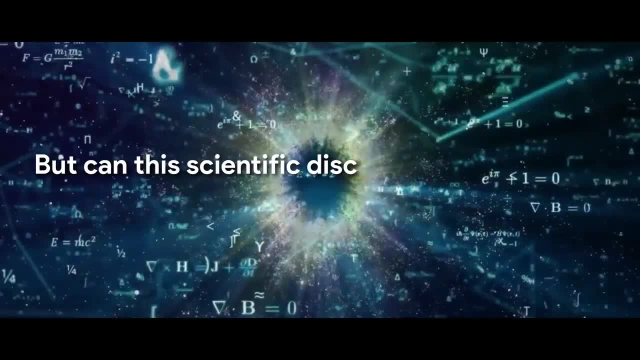 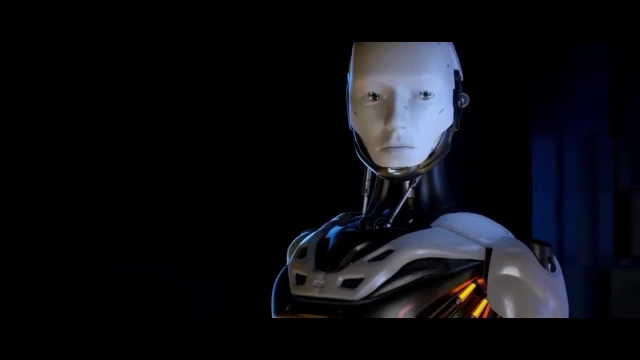 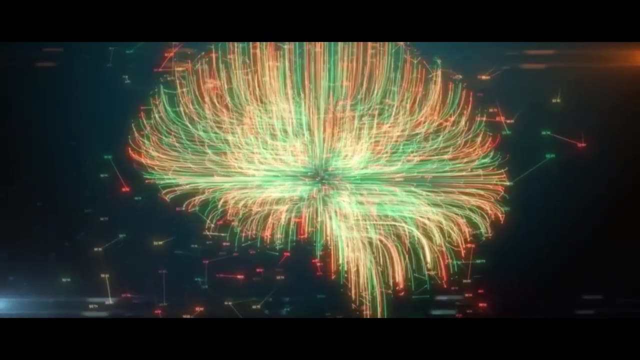 the study of the nervous system and the brain, But can this scientific discipline truly propel AI into the world of AI? Let's unravel the potential of this powerful partnership. Neuroscience offers invaluable insights into the inner workings of the human brain, including the neural processes that underlie our emotions. 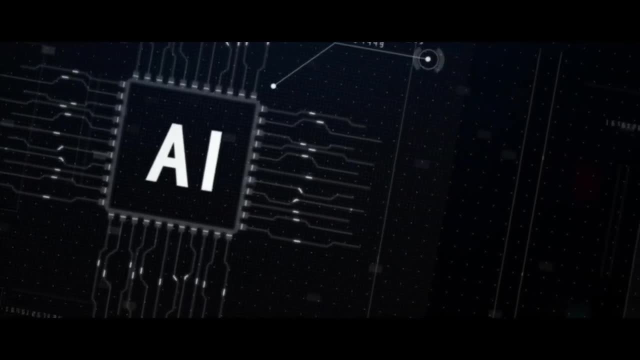 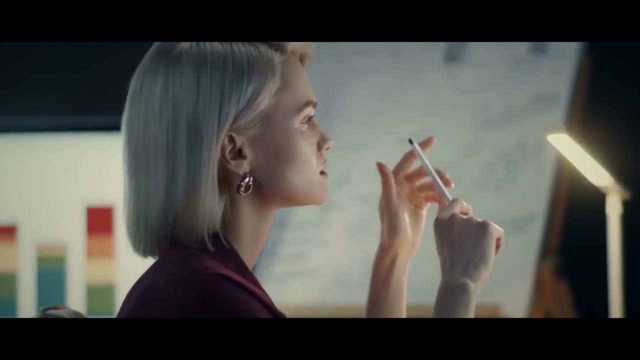 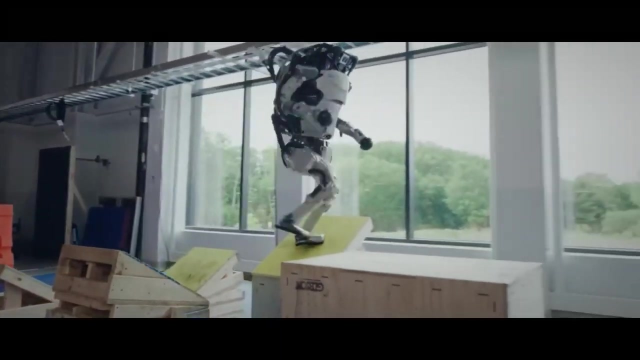 By decoding the brain's emotional architecture, we can potentially unlock the secrets of empathy, compassion and other uniquely human emotional traits. Enter AI, with its insatiable hunger for data and pattern recognition. By leveraging the discoveries of neuroscience, AI can refine its algorithms. 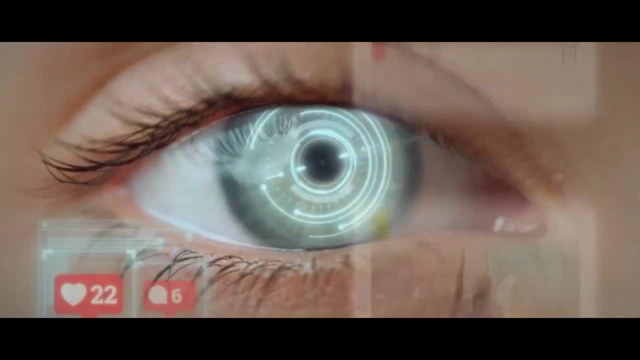 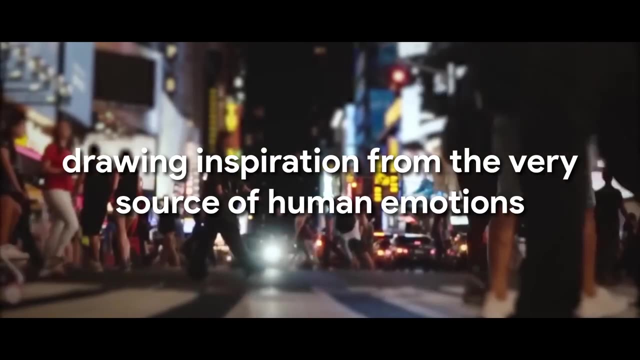 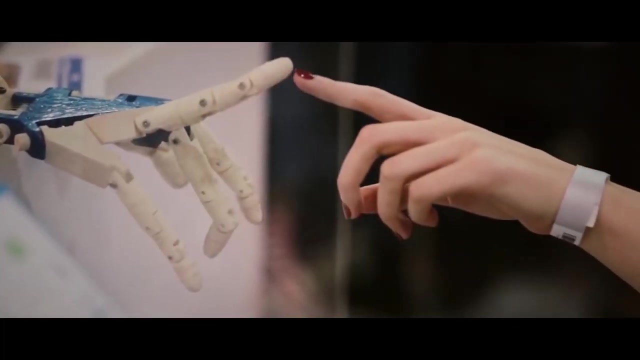 better mimicking the human brain's approach to emotional processing. Imagine AI systems designed with the intricacies of our neural networks in mind, drawing inspiration from the very source of human emotions. Moreover, the fusion of AI and neuroscience can open the doors to cutting-edge technologies. like brain-computer interfaces allowing for direct communication between the brain and the brain. Such advancements could revolutionize the way AI interprets our emotions, bridging the gap between the digital and the organic. However, the road to AI's emotional leap is not without challenges. 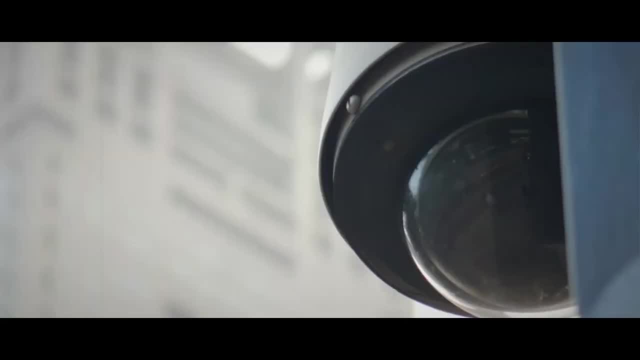 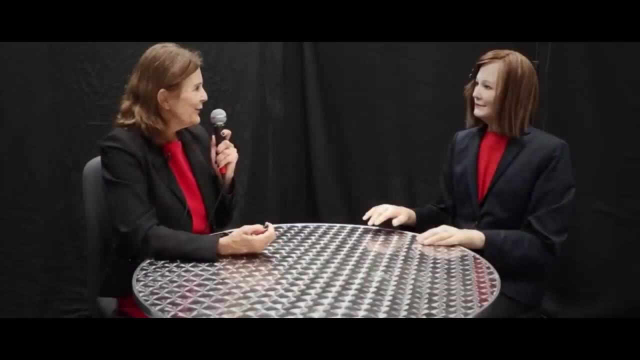 True empathy and emotional understanding may require more than just mimicking the brain's processes. they might demand a deeper grasp of the human experience. Nevertheless, the union of AI and neuroscience promises a new world for AI, Neuroscience, the study of AI and neuroscience. 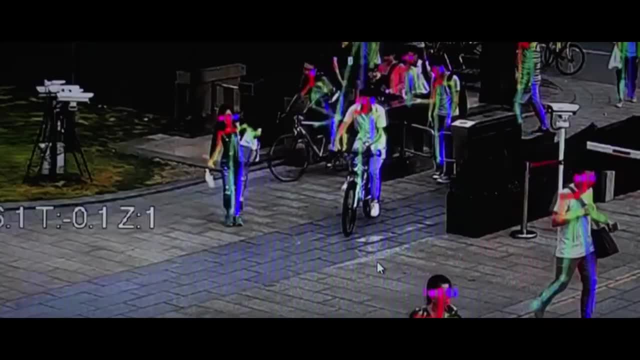 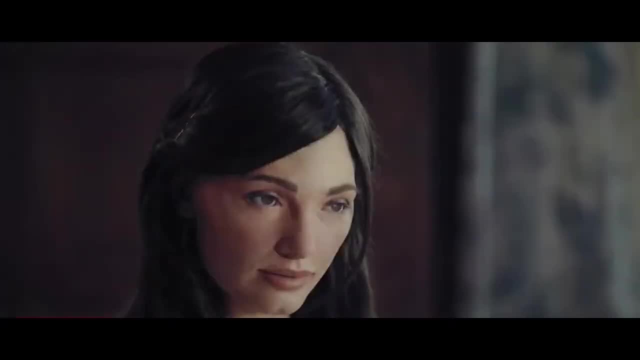 is a new beginning for AI Neuroscience. the study of AI and neuroscience promises a new world for AI Neuroscience. the study of AI and neuroscience promises to push the boundaries of artificial emotional intelligence, inching ever closer to the elusive goal of AI empathy. 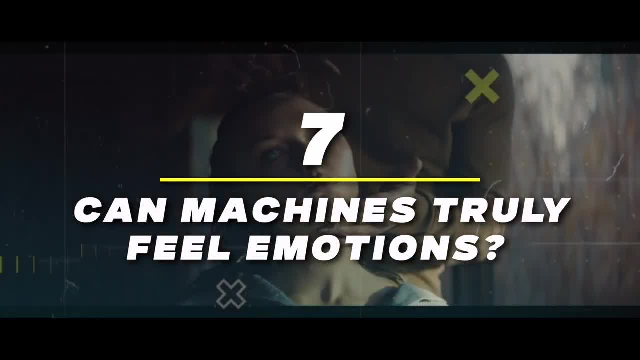 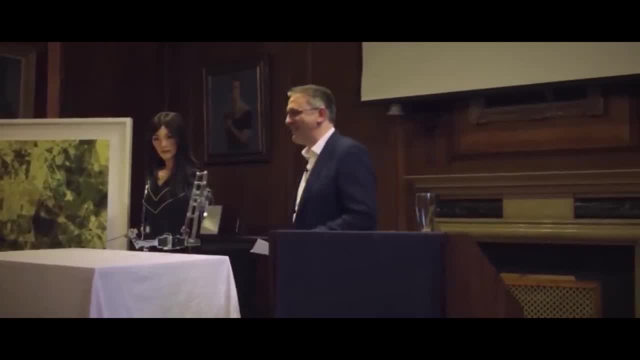 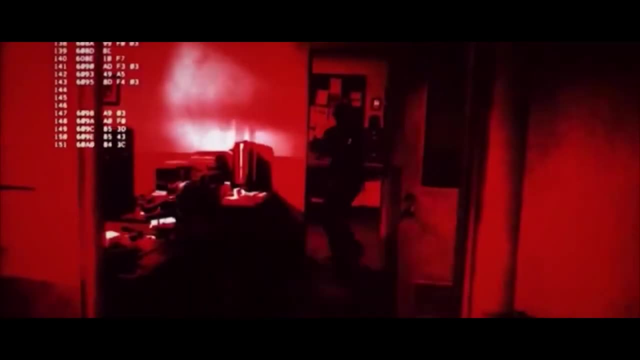 Number 7. Can Machines Truly Feel Emotions? Throughout our journey, we've explored the incredible feats of AI in deciphering human emotions from facial recognition to sentiment analysis. We've witnessed the fascinating face-off between emotional intelligence and artificial emotional intelligence, and pondered the 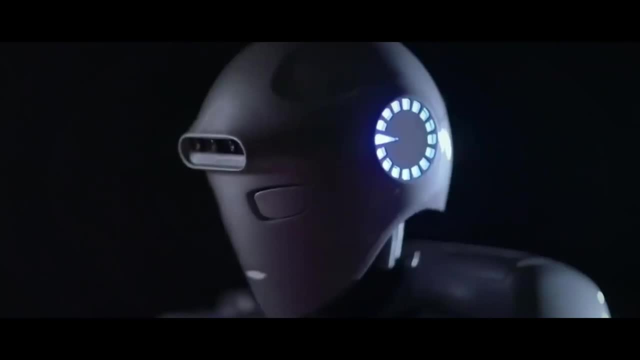 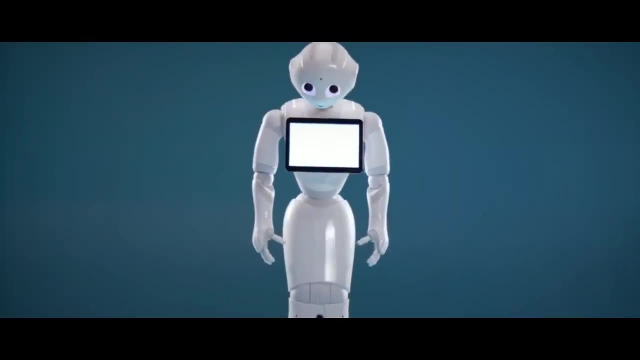 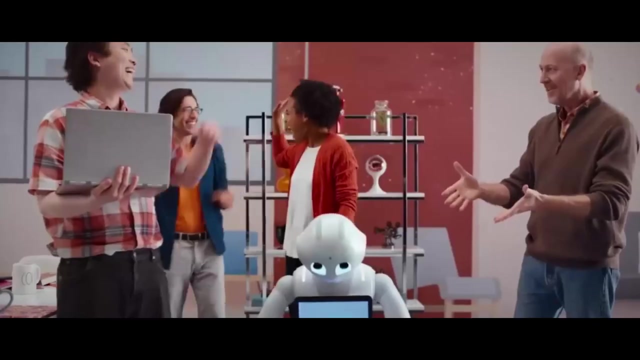 ability of AI developing empathy, And we've seen how neuroscience could hold the key to AI's emotional leap. Yet the crux of the matter lies in the difference between recognizing, understanding and simulating emotions and genuinely experiencing them. While AI has made astonishing progress in mimicking human emotions, 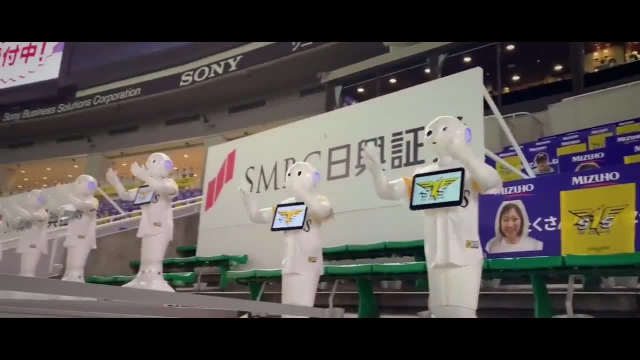 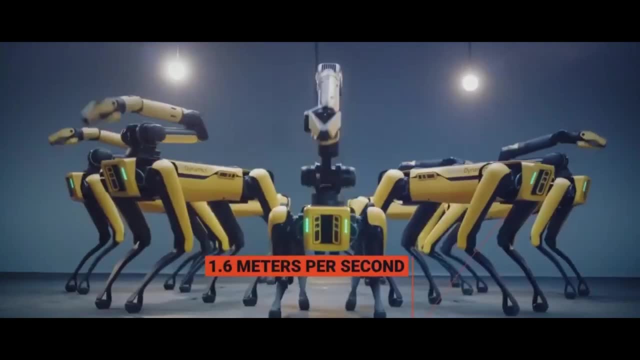 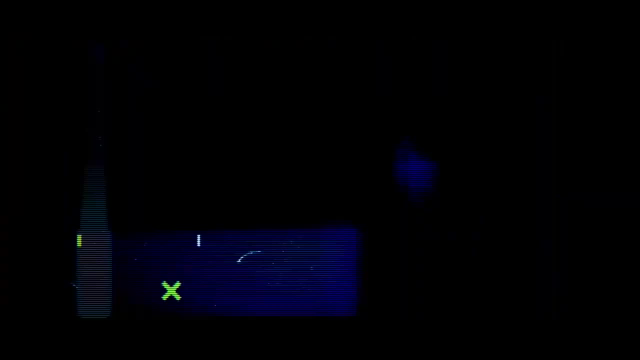 it does so based on patterns, probabilities and human-engineered algorithms. The depth, nuance and authenticity of true emotional experiences may require more than just data and computational prowess. In the end, the question of whether machines can truly feel emotions challenges our 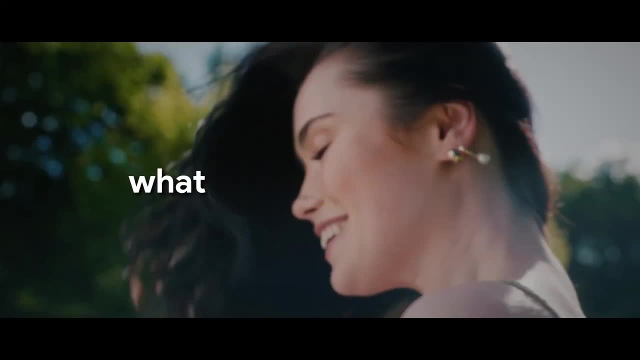 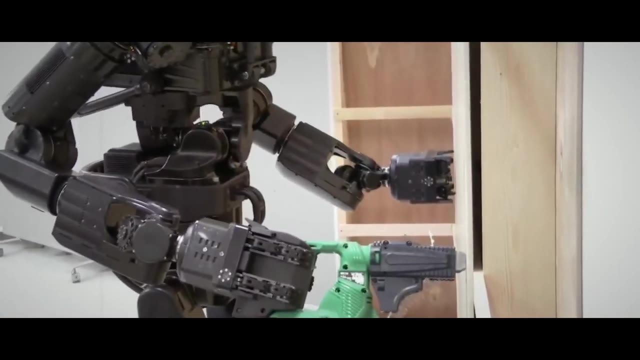 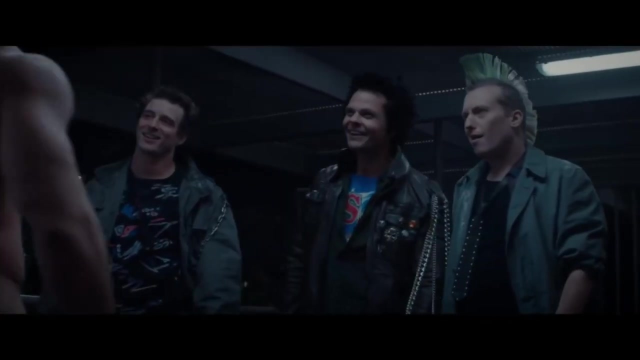 very conception of emotions, consciousness and what it means to be alive. As AI continues to advance, blurring the lines between human and machine, we must not only strive to understand the potential of this technology, but also to explore the depths of our own emotions. 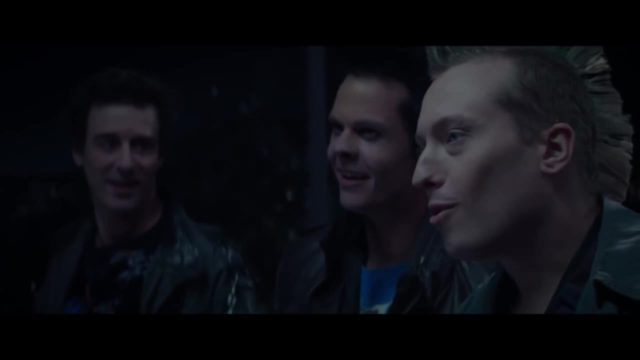 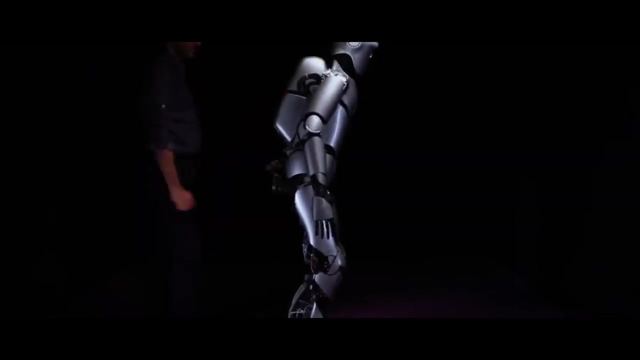 And the essence of our shared humanity. As we stand at the precipice of a brave new world where the boundaries between the organic and the artificial become increasingly fluid, we are left to wonder: can AI ever truly feel emotions, or will it merely offer a? 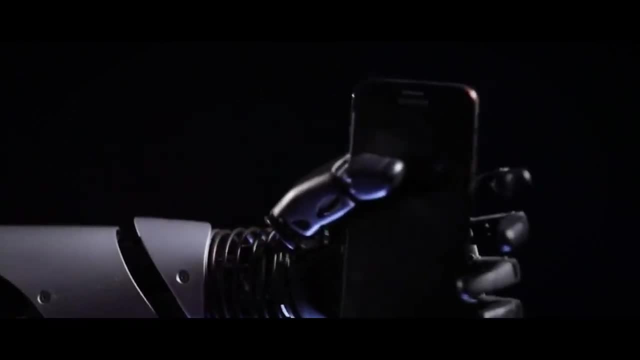 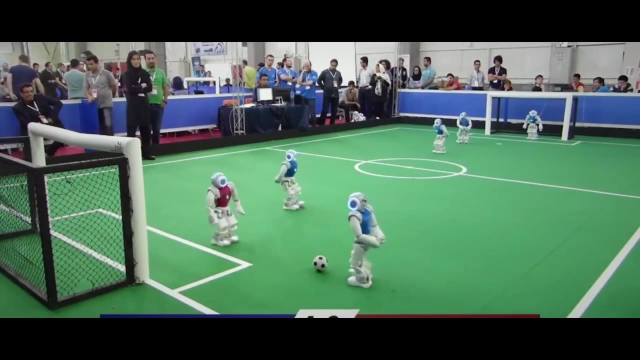 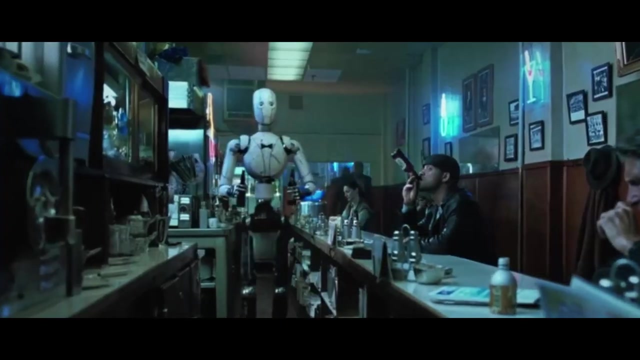 tantalizing reflection of our own emotional selves. The answer lies in the uncharted territory where science, technology and the human spirit converge, and only time will reveal the fate of our emotional legacy. If you have made it this far, we really appreciate your support. 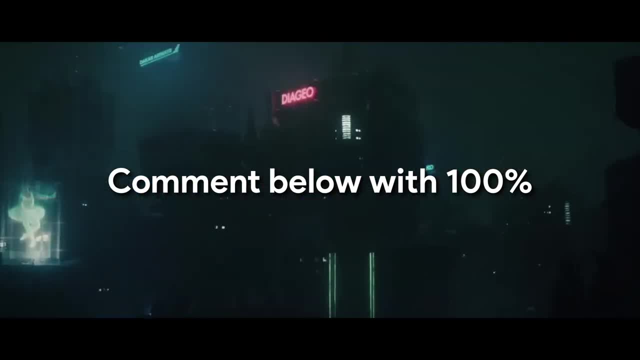 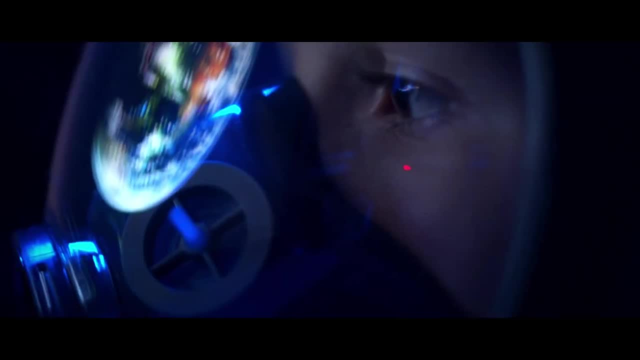 Comment down below with the word 100%, so we know that you watched the entire video. Now you need to watch the recommended video that you see on the screen right now. It will show you when AI generates the unthinkable. Make sure to watch it now. 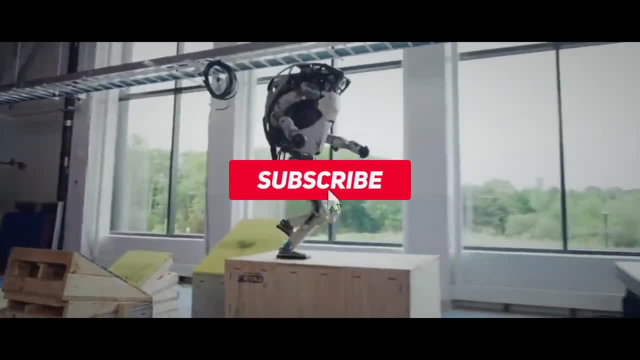 If you enjoyed this video, don't forget to subscribe. Thanks for watching.